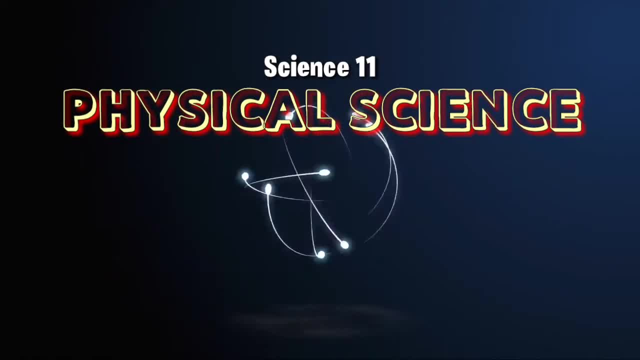 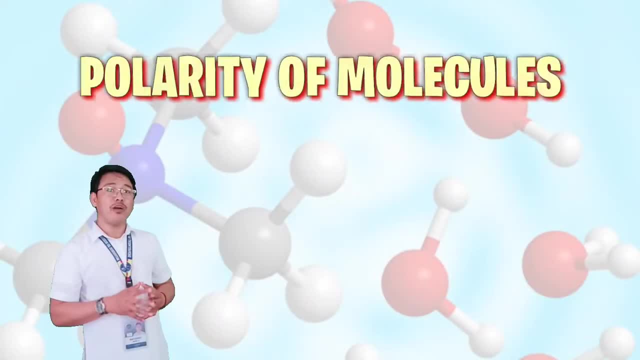 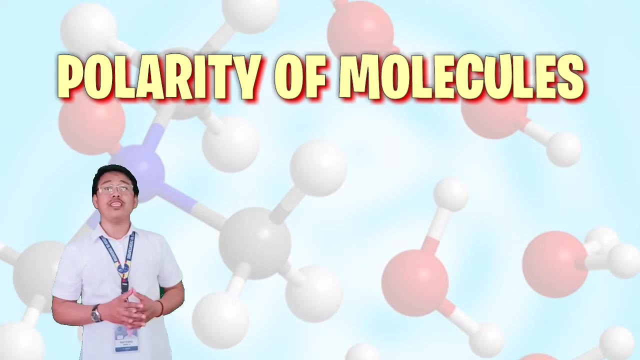 Hello Brain11, welcome to our physical science class. Today you will learn about the polarity of molecules. We will try to understand the difference between the two types of molecules according to polarity: the polar molecules and the non-polar molecules. At the end of this video, you should be able to determine if a molecule is polar or non-polar. 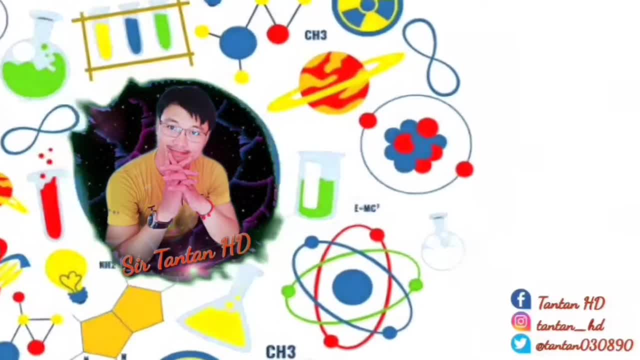 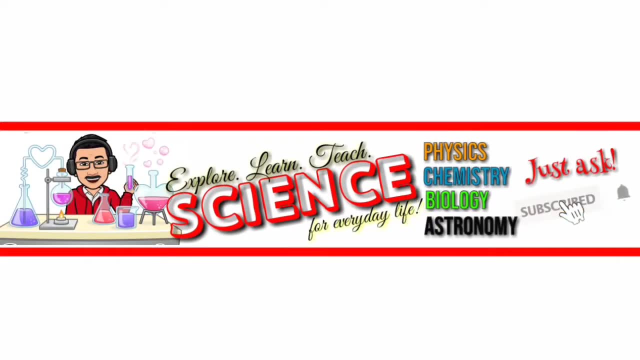 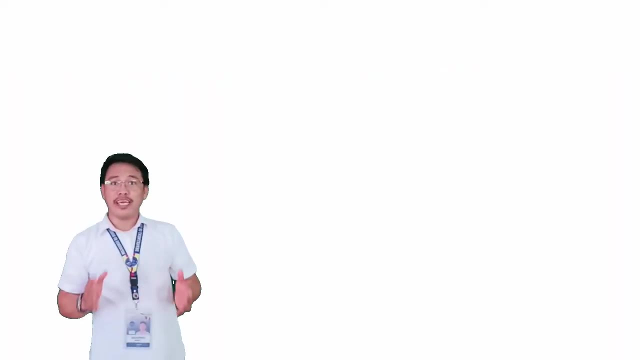 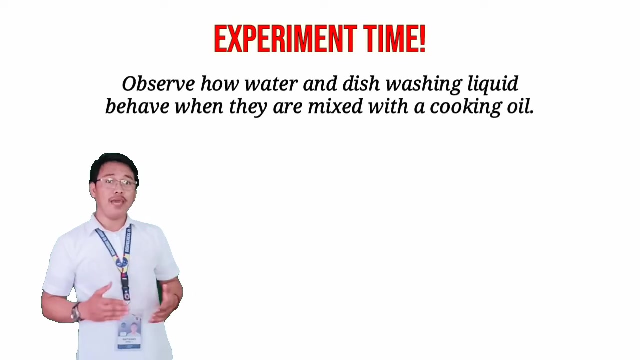 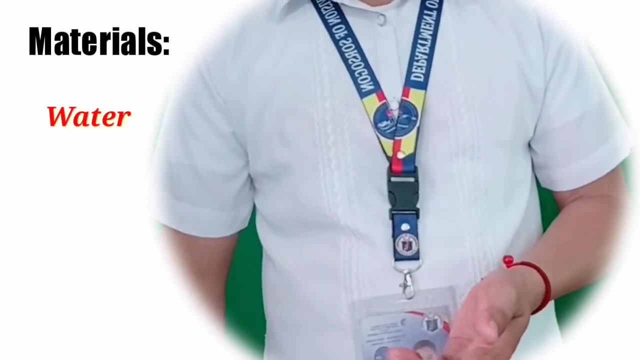 For today's lesson. let's do this simple experiment first. We will observe how water and dishwashing liquid behave when they are mixed with a cooking oil. To do this, we will be needing a water, A cooking oil, a dishwashing liquid and a steering rod. 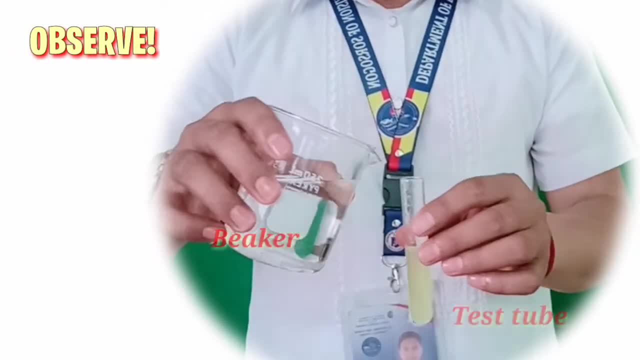 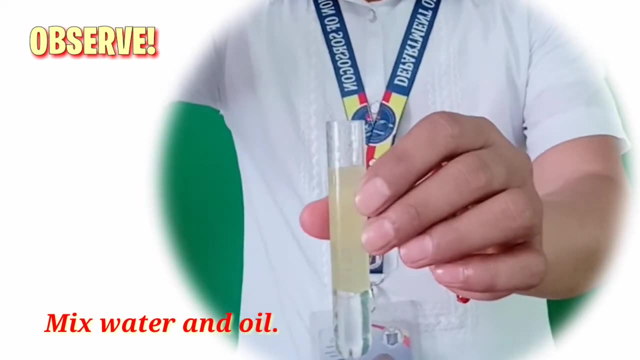 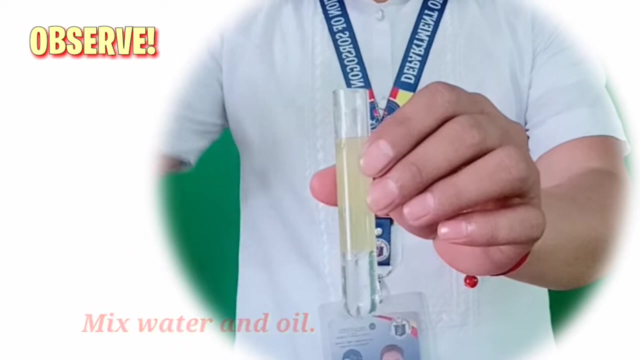 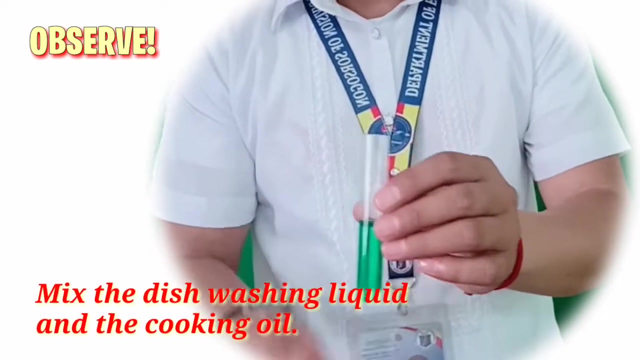 Let's do it First. let's put water and cooking oil in a test tube, Then mix. What do you notice? The water and cooking oil will never mix. Now let's try the dishwashing liquid and the cooking oil. Let's see. 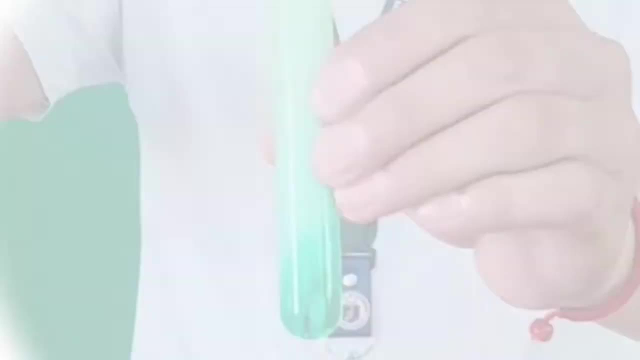 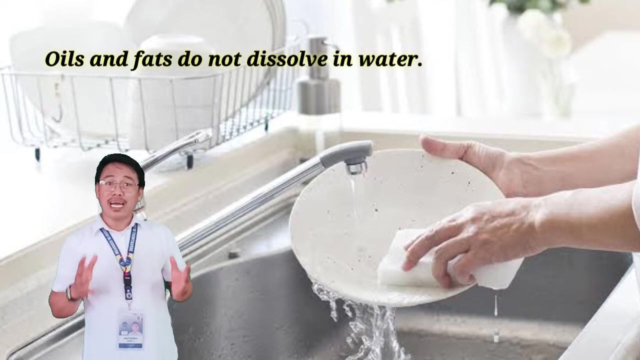 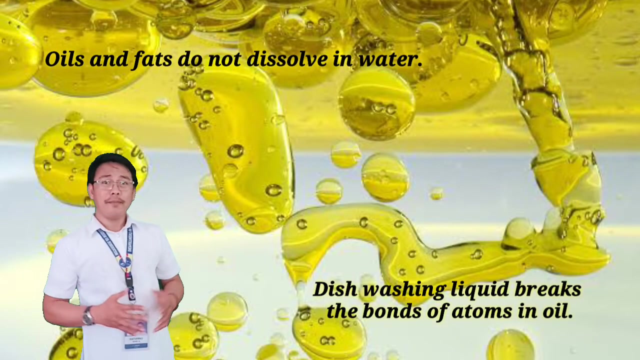 See, They're mixed together. In this simple experiment. we will know that we cannot wash dishes only with water. We will need a dishwashing liquid because the oil is not dissolving. But why? That is what we will study in this video. 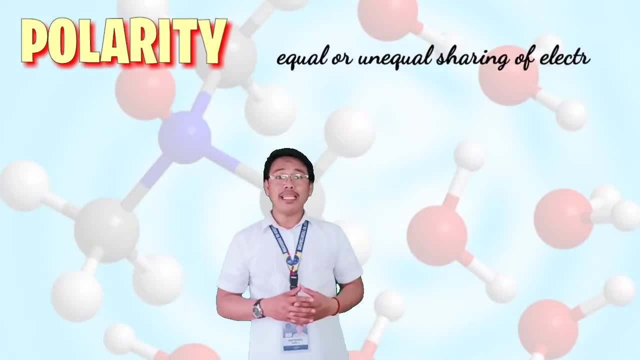 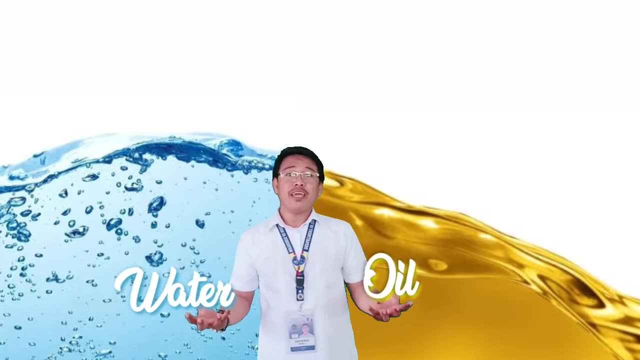 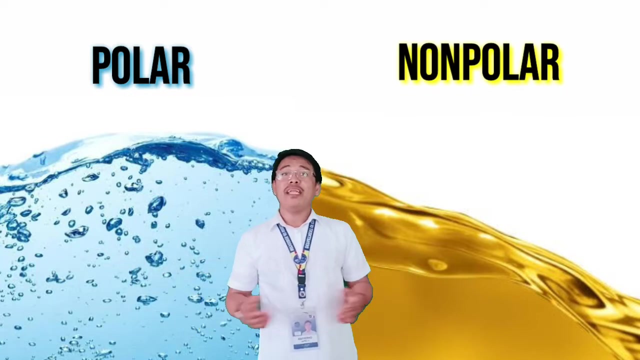 Polarity happens when there is equal or unequal sharing of electrons among the atoms of a molecule. In the case of water and oil, they will never mix, because water is a polar molecule, while oil is a non-polar molecule. Now let's take a closer look at how these two types of molecules differ. 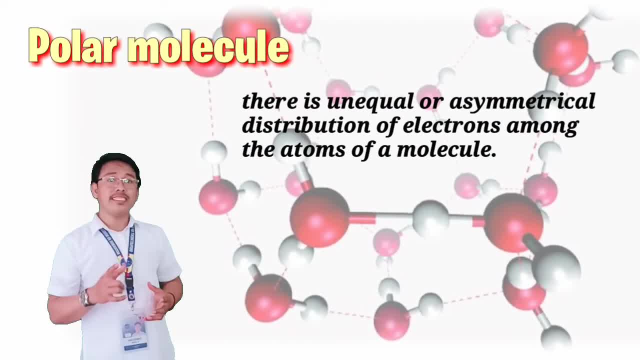 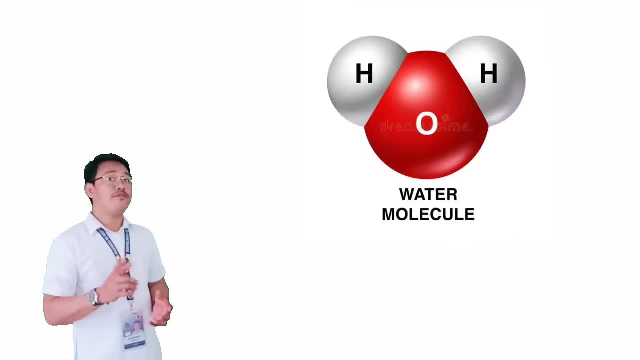 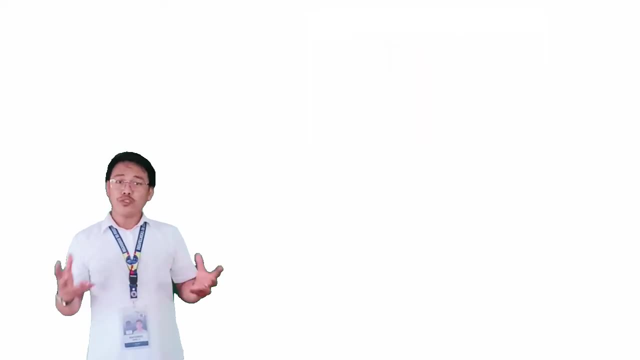 A molecule is said to be polar when there is unequal or asymmetrical distribution of electrons. What does this mean? Water, for example, is a molecule composed of two hydrogen atoms and one oxygen atom. If we are going to draw the molecular structure of oxygen atom, 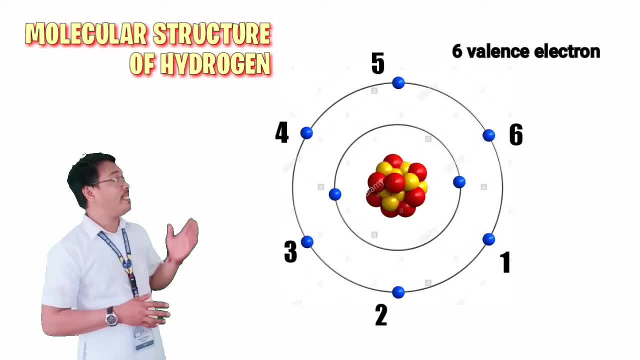 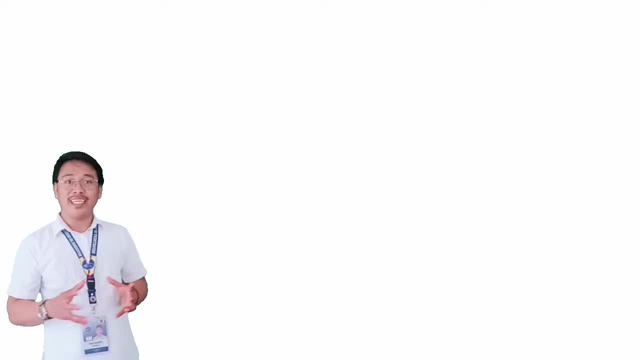 you will notice that it has only six electrons in its atom And it has only one electron in its shell. We call this the valence electron, As discussed when you were in Grade 9,. Octet Rule states that atoms tend to gain, share or transfer electrons. 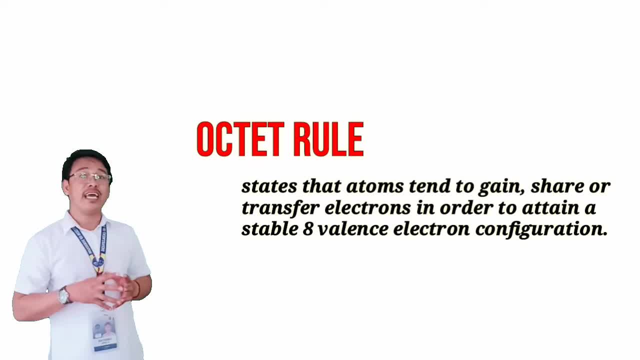 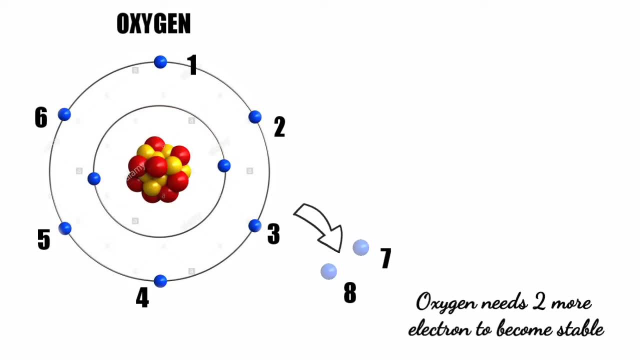 in order to attain a complete set of valence electron configuration. Therefore, oxygen needs two more electrons to become stable. Hydrogen, however, is an exemption to the rule, since it has only one electron in its shell. To become stable, hydrogen needs one more electron. 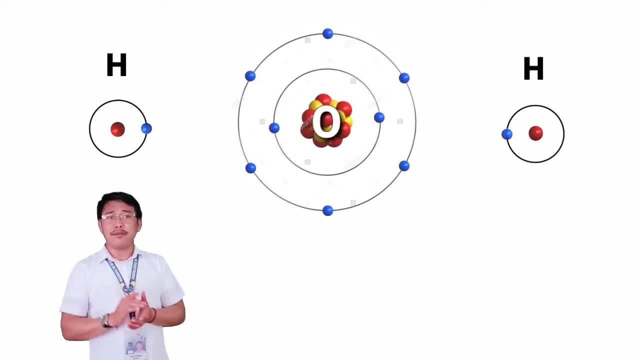 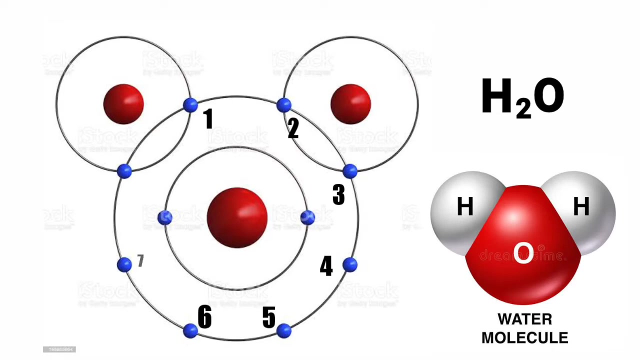 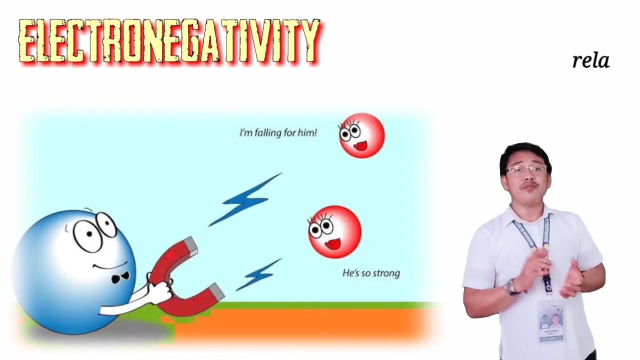 Now, since they both need electrons to become stable, they will share electrons with each other. Oxygen will share its electron to hydrogen and hydrogen to oxygen, forming water molecule. Oxygen now has eight electrons and hydrogen has two, making each atom stable. Now, this relative ability of an atom to draw electrons in a bond toward itself, 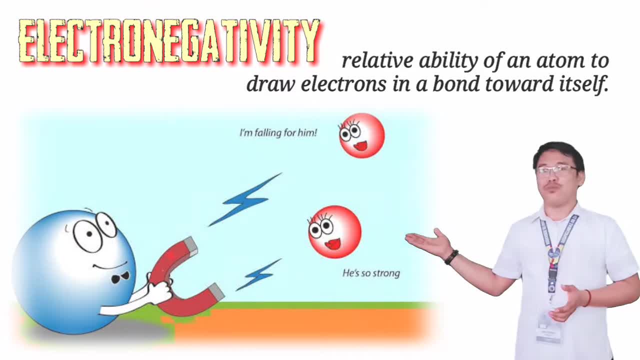 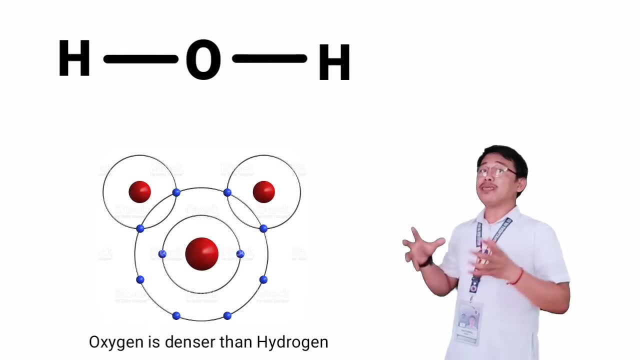 is called electronegativity of the atom. Because electrons have more or denser oxygen compared to hydrogen, its electronegativity, or its ability to attract electrons, becomes higher, giving it a partial negative charge. On the other side, hydrogen has a lower electronegativity. 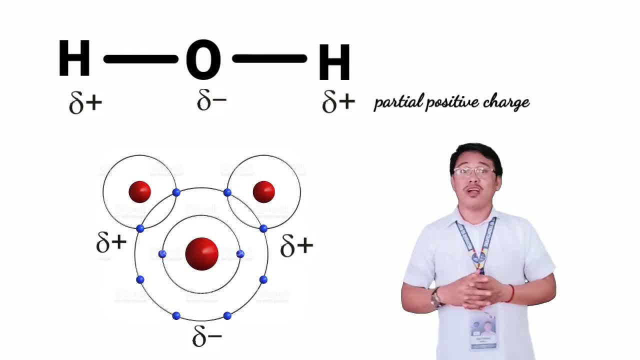 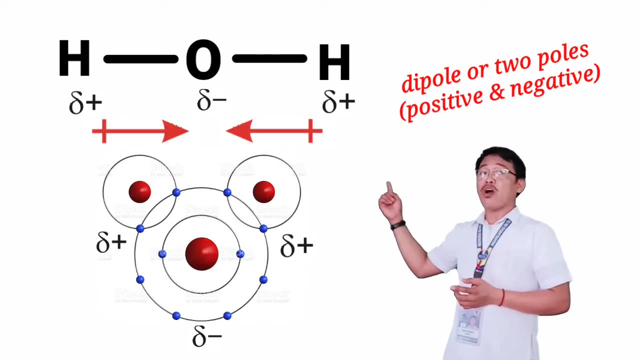 which is why it has a partial positive charge. This unequal sharing of electrons between atoms creates a dipole moment, or two poles: the positive and the negative. We will represent this with an arrow pointing towards oxygen, since oxygen is more electronegative than hydrogen. 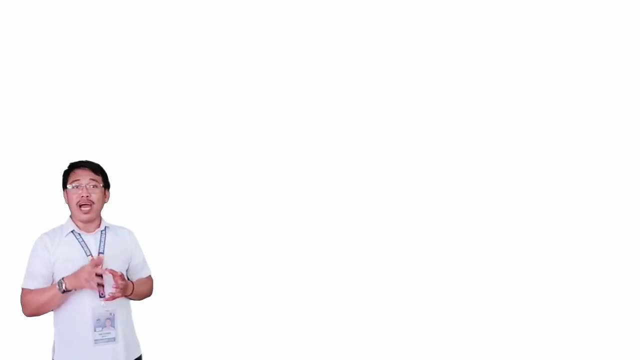 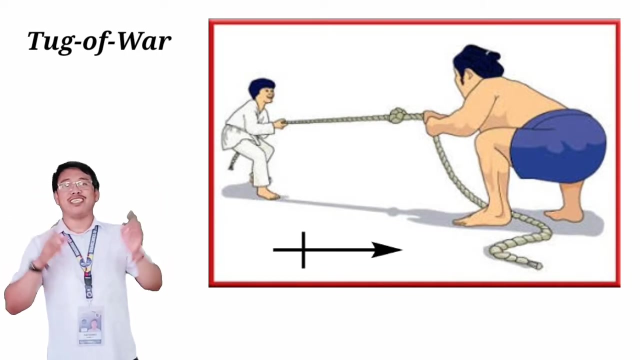 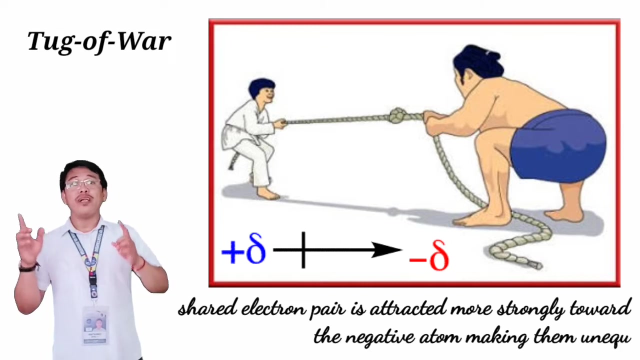 The sharing of electrons by two atoms may be likened to a tug-of-war between two men. The stronger man drags the other across a central line Between atoms. the shared electron pair is attracted more strongly toward the negative atom, making them unequal or asymmetrical, creating a polar band. 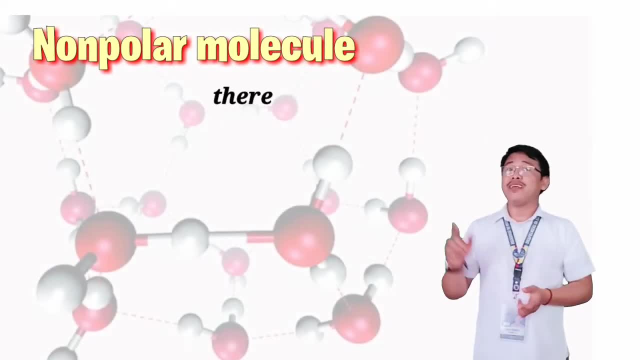 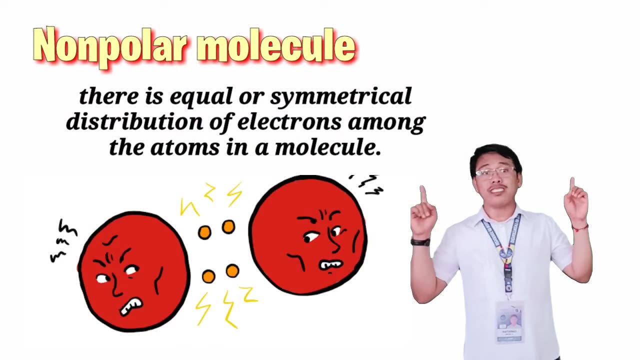 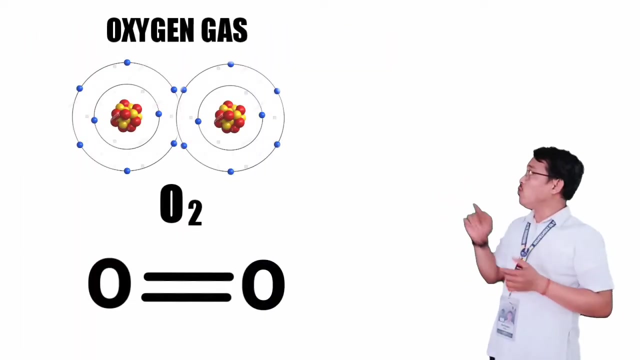 Nonpolar molecules, however, are formed when there is equal or symmetrical distribution of electrons. This happens when the bonding atoms have approximately equal ability to attract electrons on each side. Let's have oxygen, gas, O2, as an example. As we had discussed earlier, oxygen has six valence electrons. 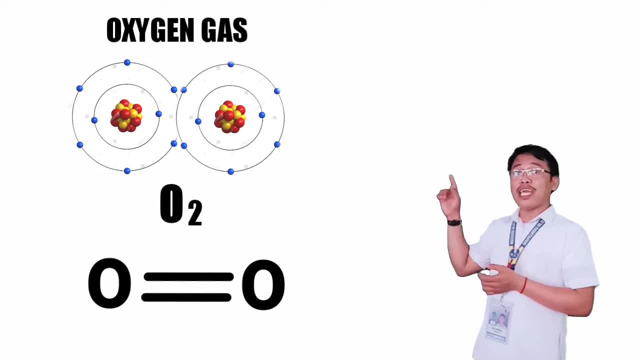 So when two oxygen atoms with the same electronegativity combine, what will happen? As you can see, the electron density is spread evenly between the two atoms in the band. Since a pair of electrons is shared equally between atoms, there is no partial charge created. 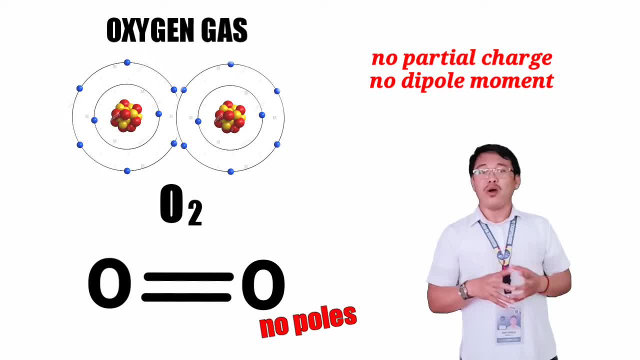 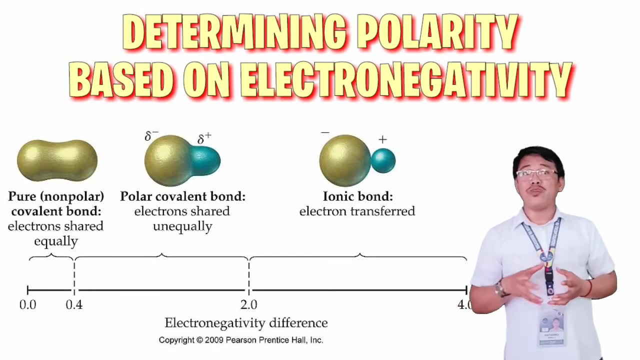 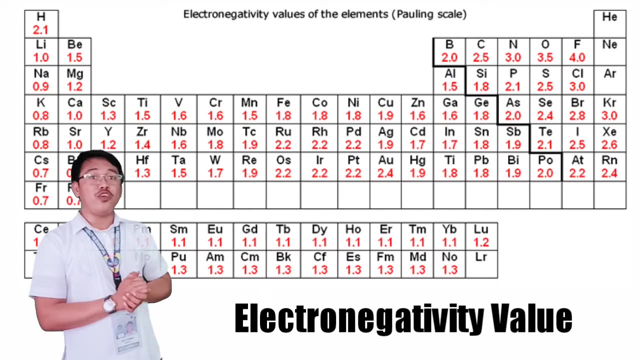 Hence no dipole moment. Therefore, oxygen gas is a nonpolar molecule. We can also determine the polarity of molecules based on the electronegativity difference between the atoms present in a molecule. To get the electronegativity value of each element we will use a periodic table. 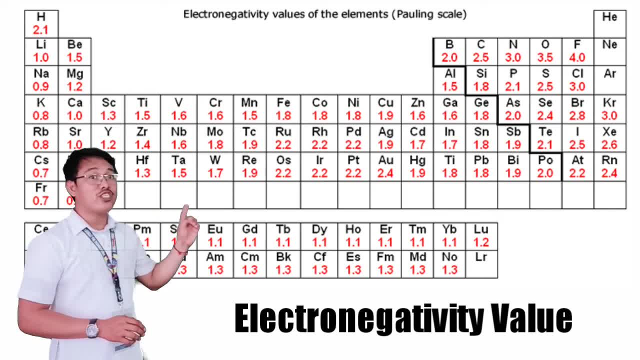 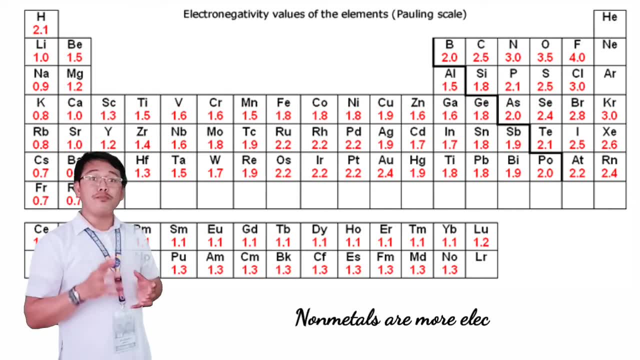 There you can see the electronegativity value of each element. Electronegativity value increases from left to right, which means that nonmetals are more electronegative than metals. In the table you can see that oxygen and fluorine have the highest electronegativity value. 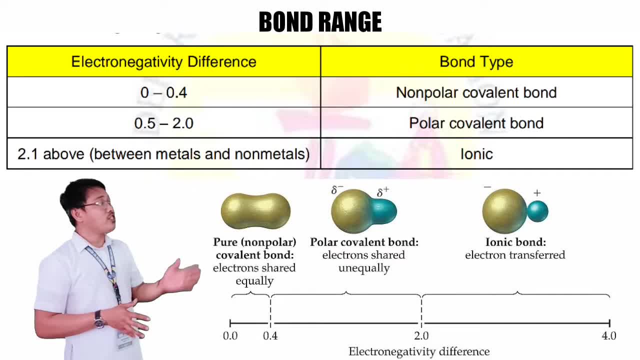 So we have to remember this band range. If the electronegativity difference ranges from 0 to 0.4, the type of band is nonpolar covalent- 0.5 to 2.0, it is a polar covalent band. 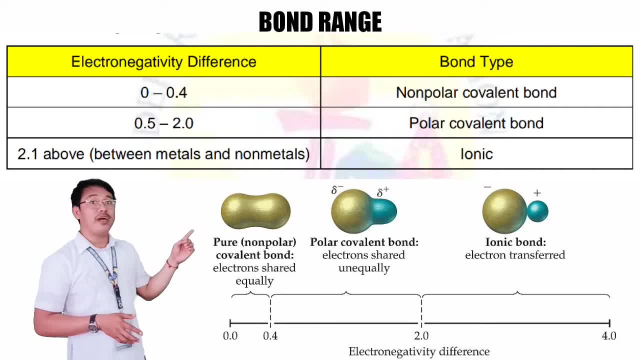 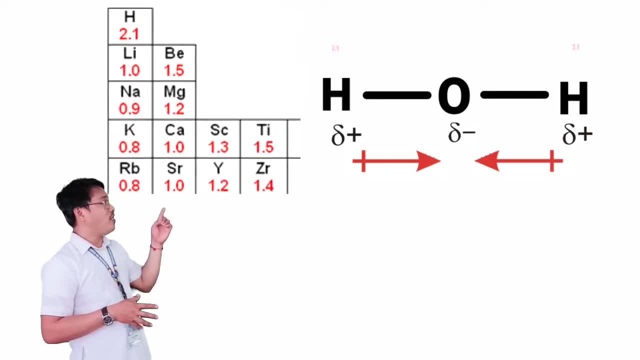 And when the value is 2.1 above, the molecule is in an ionic band. Now let's use again water as an example. The electronegativity value of hydrogen is 2.1 and oxygen is 3.5.. 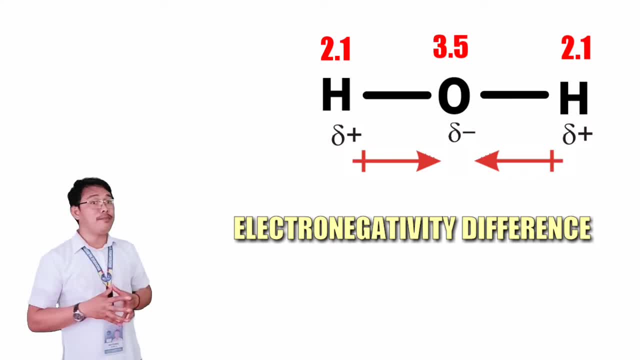 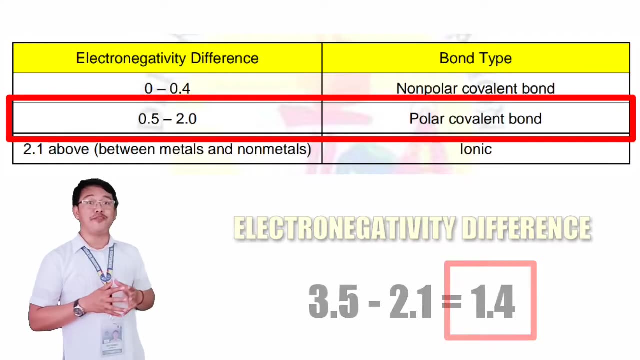 To get the electronegativity difference, we simply subtract 2.1 from 3.5. This becomes 1.4.. So since the value is 1.4 and is within the 0.5 to 2.0 band range, 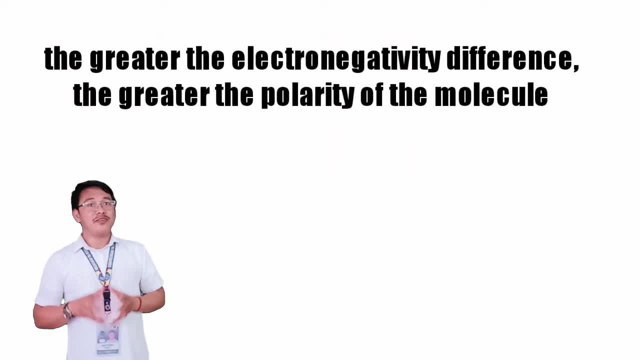 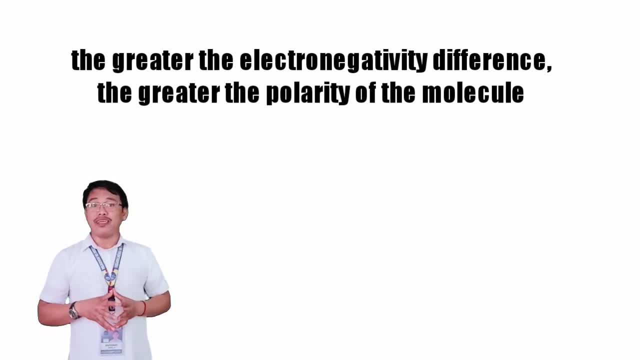 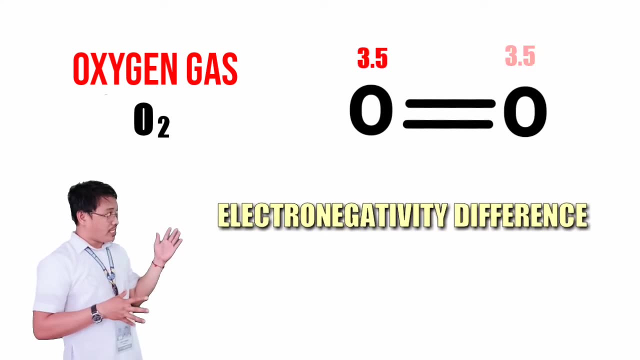 water is polar. The greater the difference between the electronegativity of the atoms involved in the band, the greater is the polarity of the molecule. For the oxygen gas, O2,, the electronegativity value of oxygen is 3.5.. 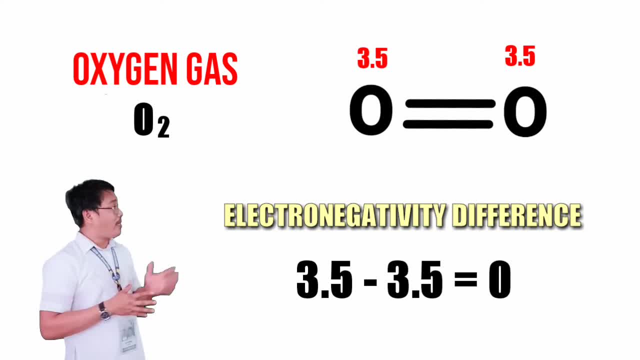 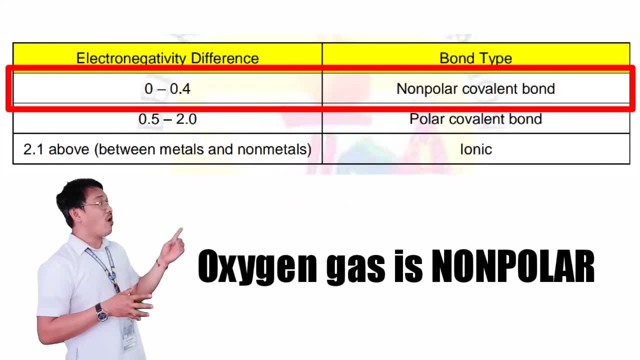 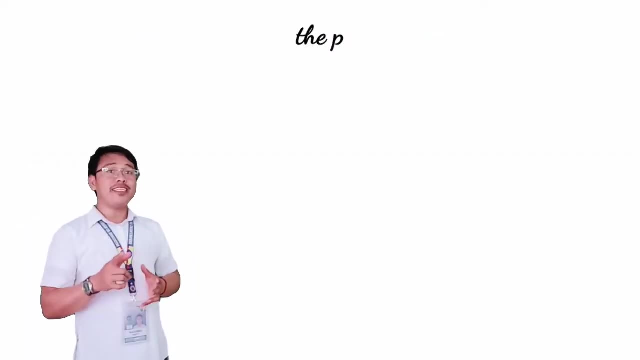 Therefore, 3.5 minus 3.5 is 0.. So this is within the band range of 0 to 0.4, which means that oxygen is a nonpolar covalent. That simple. However, the polarity of molecules do not depend solely on the type of band present. 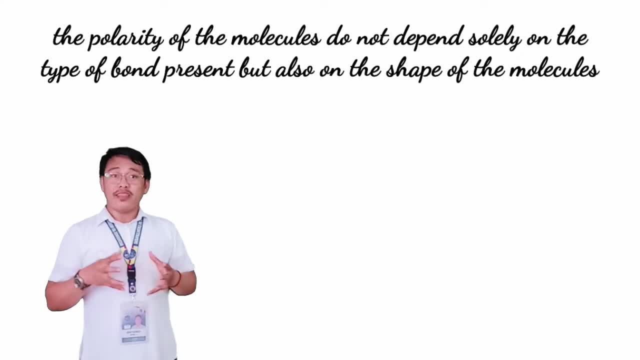 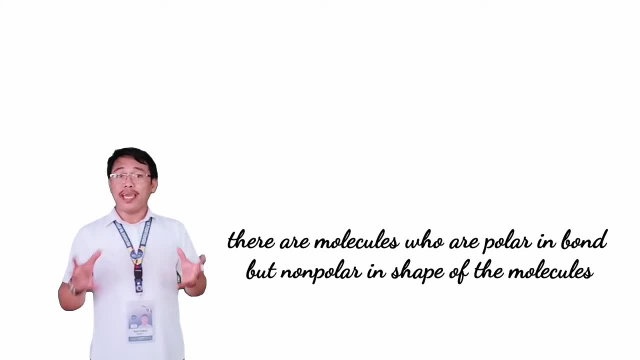 but also on the shape of the molecules. This means that there are molecules who are polar in bonding, but is actually a nonpolar molecule based on the shape of the molecules. Maybe you are now wondering how it happened. Let's use carbon dioxide as an example. 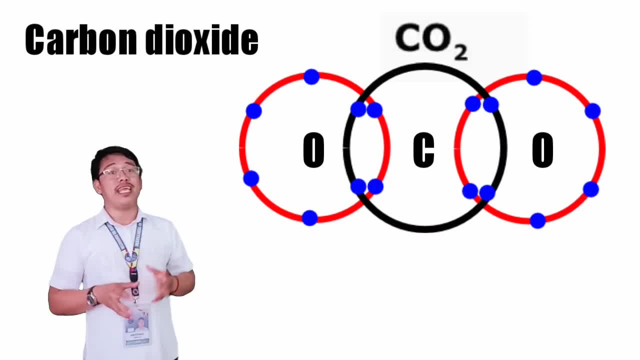 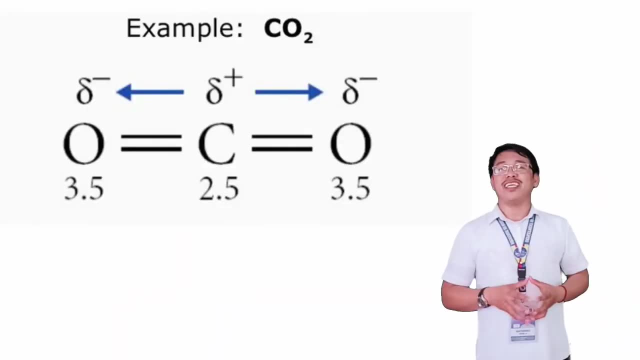 Carbon has 4 electrons and oxygen has 6.. So carbon needs 4 and oxygen needs 2 to become stable. Therefore, the 2 oxygen atoms will share its electrons to carbon, making them stable. Since oxygen is denser, it gains a partial negative charge. 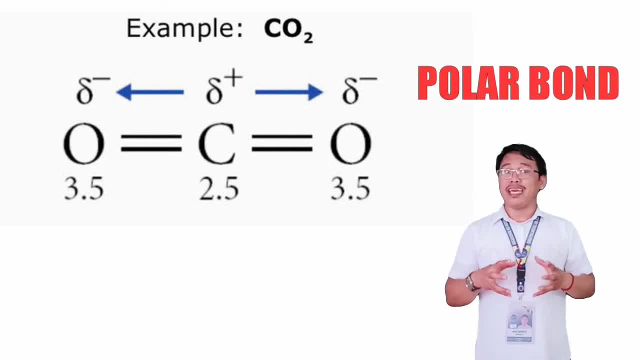 and carbon a partial positive charge, making it a polar molecule. In terms of the electronegativity, the electronegativity value of oxygen is 3.5 and carbon is 2.5, giving them an electronegativity difference of 1.0. 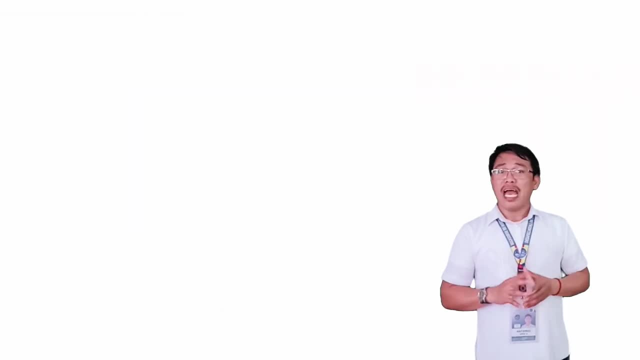 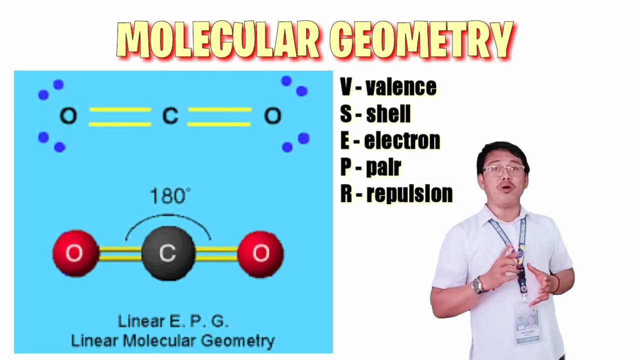 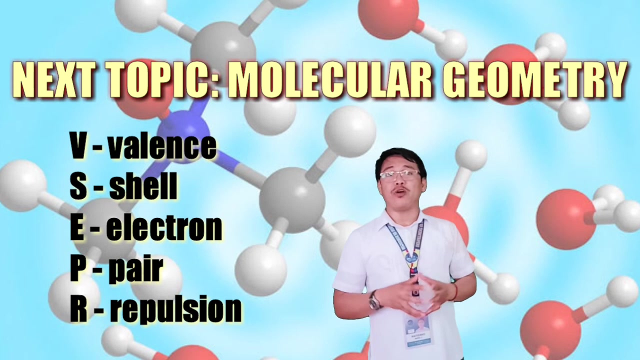 making the molecule a polar band. However, based on the molecular geometry or the shape of the molecules, carbon dioxide is a linear molecule, making it a nonpolar molecule. We will discuss this topic, about molecular geometry or the shape of the molecules, in our next video.